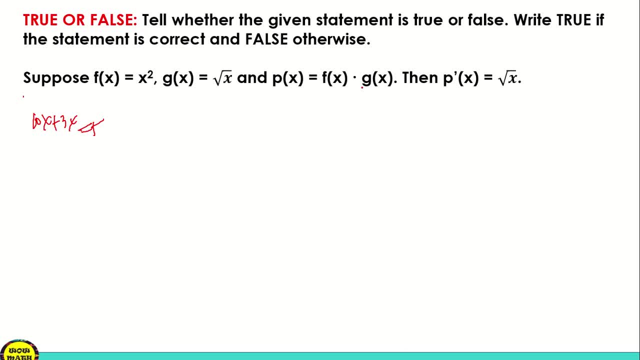 Next, Okay, number 2.. Suppose f of x is equal to x squared and p of x is equal to the product. Okay again, suppose f of x is equal to x squared, g of x is equal to the square root of x and p. 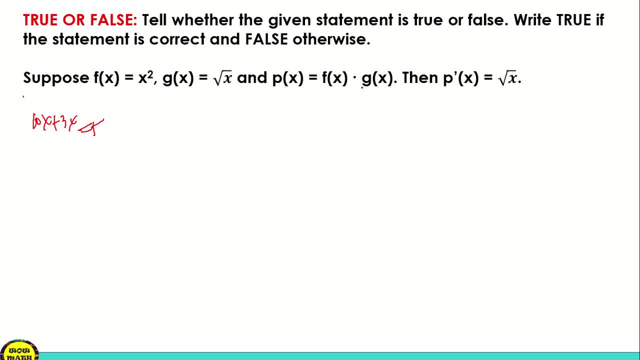 of x is equal to the product of f of x and g of x. Now we are going to get the p prime x. Okay, let us see. if the answer is square root of x, We are going to write it in this. Let us write it: Okay, so f of x is equal to x squared. 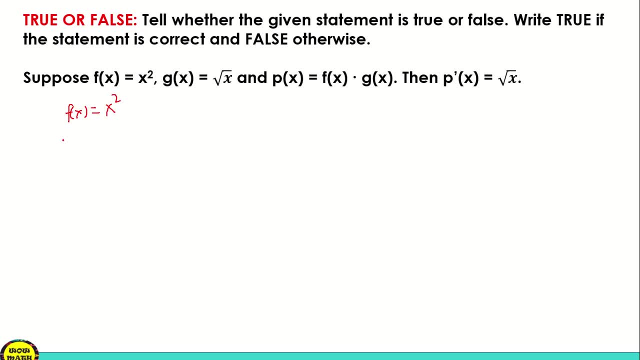 g of x is equal to square root of x And this will be okay. we write as: x raised to 1, 1 halved. okay, in the exponential form. And that p of x we will take and this is our end. So what we are going to do now is let us the right side here we are going to counselor that in the exponential form. So here at E we are going to give away. we will give away half Tú p is equal to g nating that Then, when we see it right here first we are going 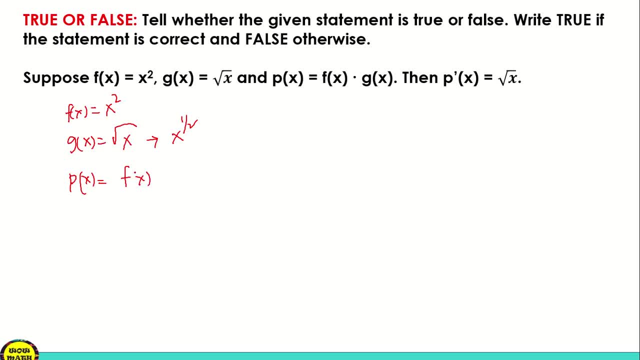 to get the value in the exponential form. So the amount of the value you are going to give up, this nating, nating, nating, you required is exactly 4.7.. And then, once you know that you have the value in, your is the product of f of x and g of x. so we're going to answer first yung p of x natin, yung. 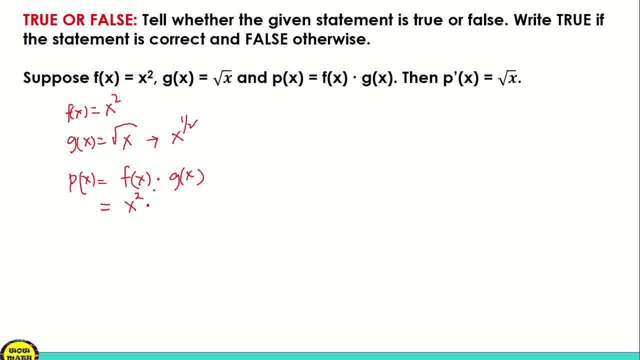 f of x natin is x squared times. okay, yung g of x natin is square root of x, so we can transform into exponential form. so that is x raised to one half. so applying yung anin natin exponent kapag nagmumultiply tayo, nagmumultiply tayo, yung exponent natin ay ina add, so that will. 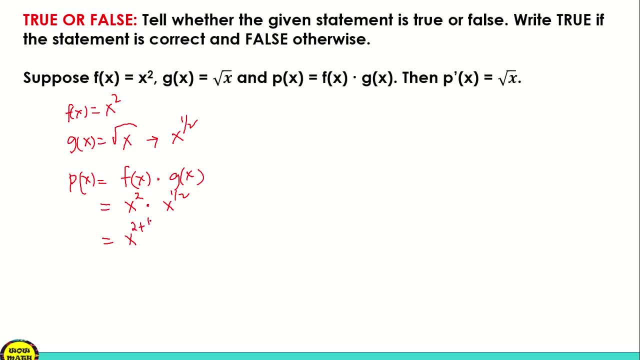 be x raised to two plus one half, and the answer is: x raised to, that is five over two. so this is the answer for p of x. now kunin daw natin yung ang sabi sa: given ang p prime of x daw natin. 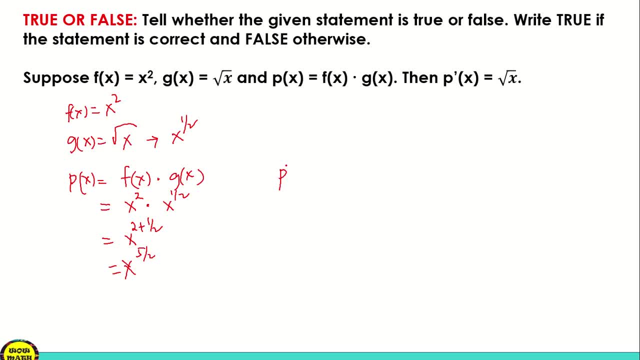 so tingin natin so p prime of x is equal to x raised to five over two. so kinukuha na natin yung derivative ng p of x natin. so now our exponent is five over two. five over two. then multiply natin yan dito sa okay, since one yung numerical coefficient pinin natin ilalagay. so copy x: 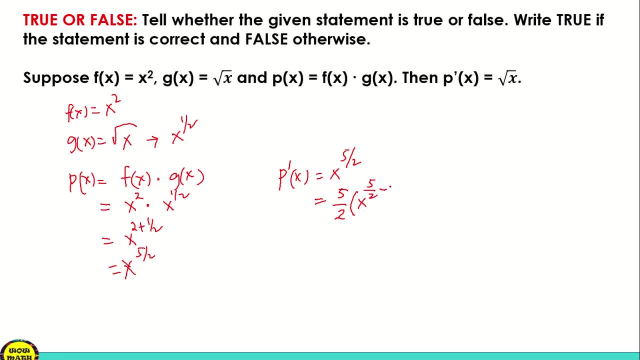 and then yung five over two natin ng isa, and then that will be five over two x raised to. okay, this is pano kayo nagsosubtract nito. so ang ginagawa pwedeng ganito: plus si two, imumultiply natin kay one. so that is negative. 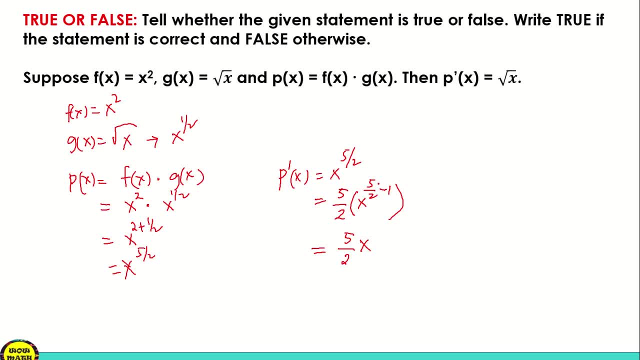 uh two, so negative. two plus five, pwedeng ganon, or five uh minus two, the answer is three. okay, same pa rin yung denominator yun, which is two. so the answer is five over two, x raised to three over two. or pwedeng natin isulat ito as paano natin isulat, pwedeng natin siyang. 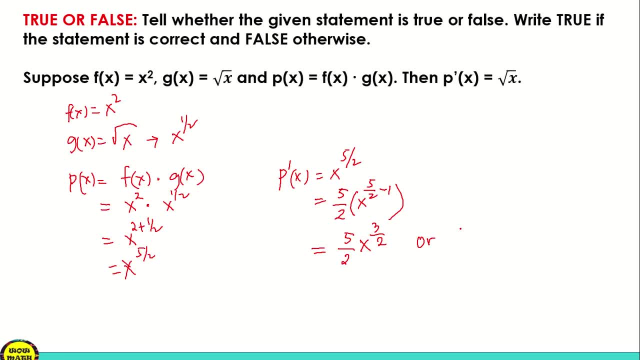 gawing or five over two, tapos gawin natin yung x natin, as that is the square root of x cube. okay. so pwedeng ganito: or five x cube over two, okay, that will be the answer. so anong sabi dito? square root of x. so ang p prime of x daw ay square root of x, pero yung nakuha 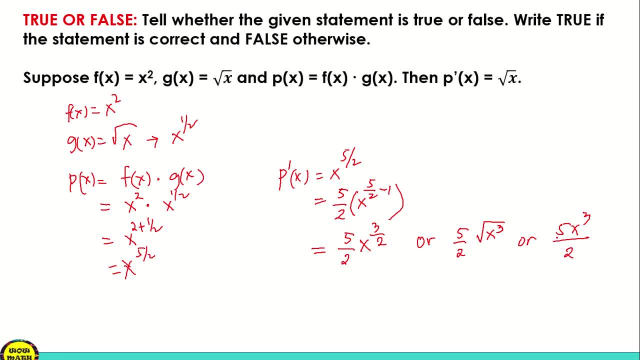 natin is five x cube ay five square root of x cube. oh, bakit ito? okay, so dapat five x cube pala. sorry, this is five x cube, nakalimutan ko. five x cube over uh five and the square root of x cube. ayusin lang natin. so para maayos, hindi lang okay. 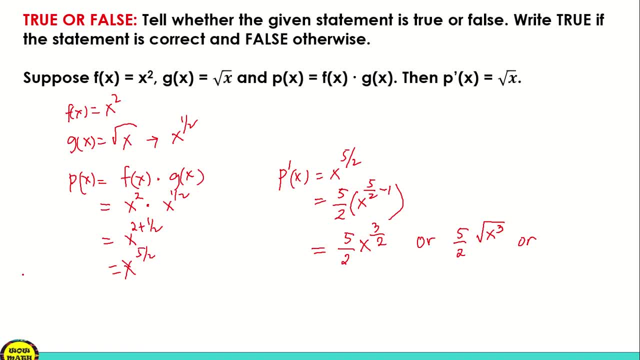 okay, ulitin natin. so pwedeng natin isulat as ganito: no five square root of x cube over two, since itoyon sagot sa p prime of x in that square root of x and therefore this statement is false. okay, next, 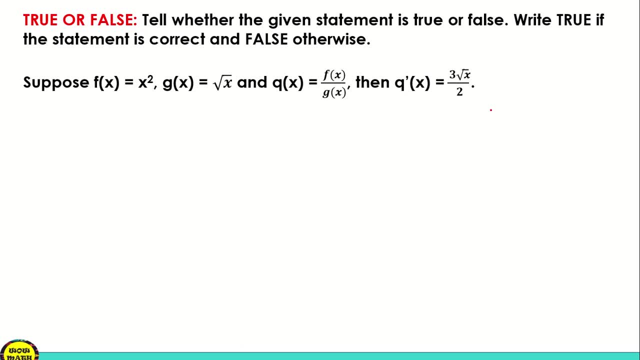 okay, suppose, uh, square root of f of x is equal to x squared. so let's put it: f of x is equal to x squared, g of x is equal to the square root of x. or you can transform that as x squared raised to one half, Now yung Q of X. 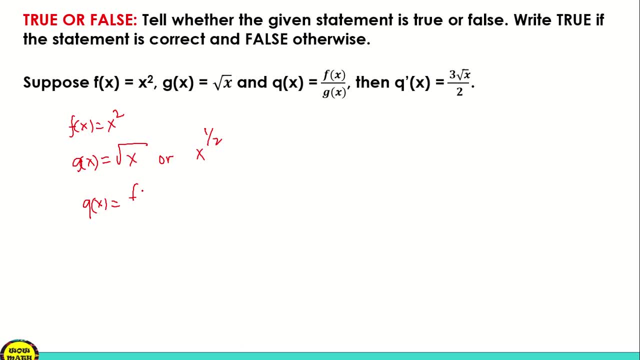 daw natin ay equal to the quotient of F of X and 3X. So what we're going to do, class, ay kunin muna natin yung value ng Q of X, So yung F of X natin is X. 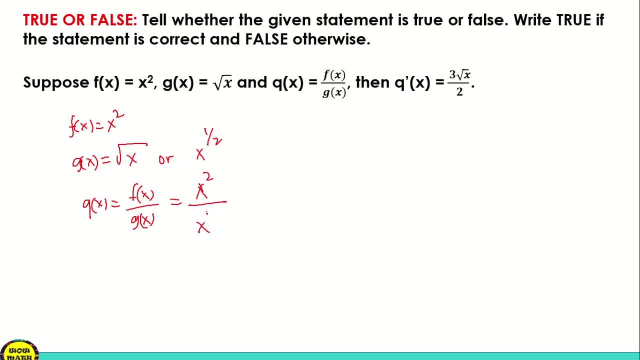 squared and then dito X raised to one half. So we all know dun sa rule ng exponent natin kapag nagdi-divide tayo. So anong ginagawa Sino-subtract natin, yung exponent? So copy lang yung base. 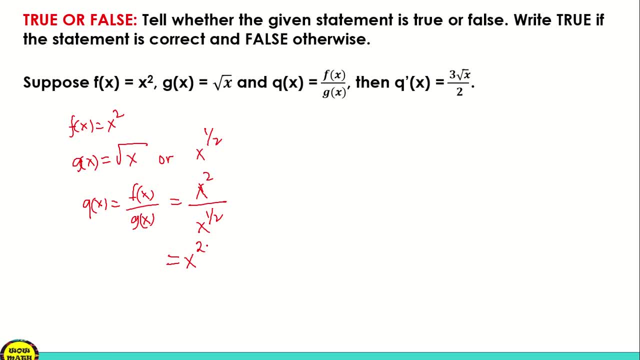 which is X, and then subtract natin yung exponent 2 minus one half, Of course. ibig sabihin yan one and one half, or 3 over 2.. Okay, paano yan Pwede ganito 2 times 2.. 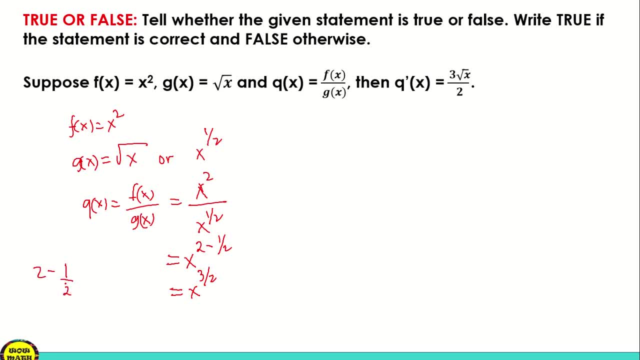 Ganito yan diba 2 minus one half, So pwede ganito gawin yan. So the answer is 3 over 2.. So X raised to 3 over 2.. So this is the Q of X. 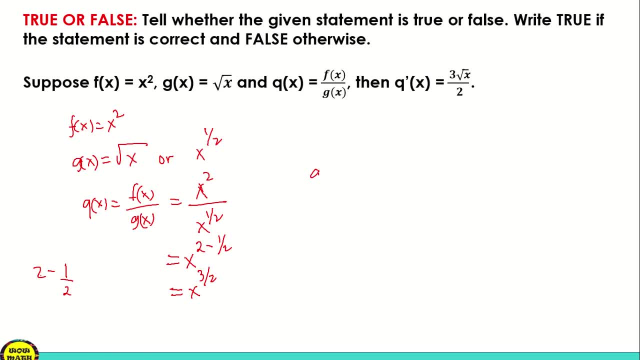 Now kunin natin yung derivative ng Q of X. So Q prime of X is equal to X raised to 3 over 2.. So what we're going to do, Multiply natin si 3 over 2 kay X, and then si 3 over 2 na exponent. Bawasan natin ang isa. 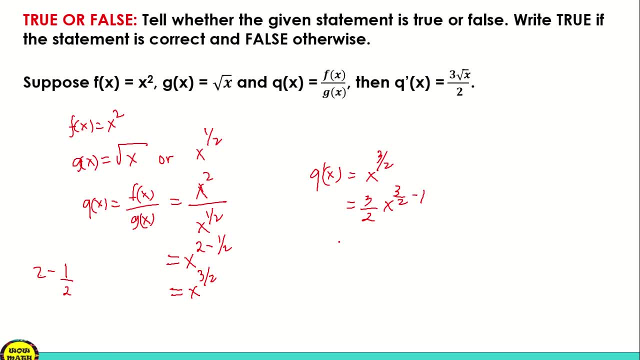 So 3 over 2 minus 1, the answer is 3 over 2.. So pwede ganito: 2 times 1 is 1.. So 2 times 1 is 2.. 3 minus 2, the answer is 1.. 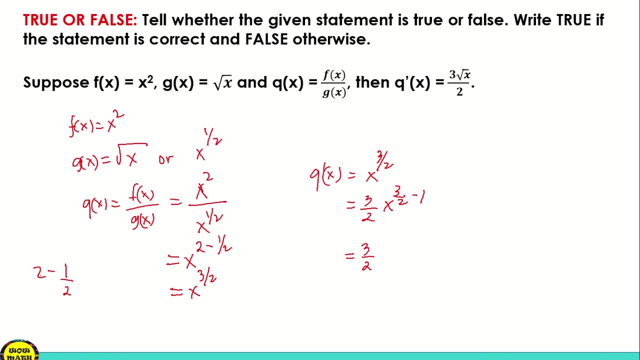 Okay, so anong sagot dito? Kasi ang 3 over 2 is 1.5.. 1.5 minus 1.. So the answer is 0.5.. Or 3 over 2, X raised to 1 half. 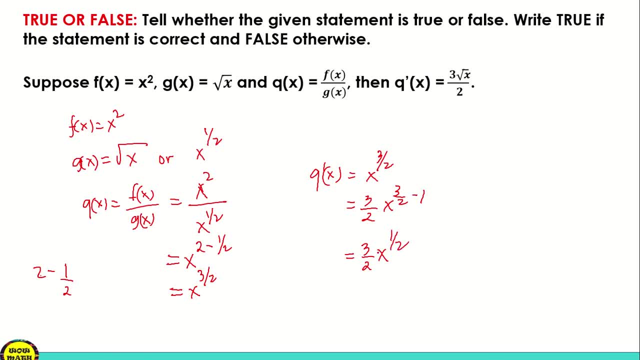 Okay so paano natin ano pa yung ibang para na pwede. ang sulit natin is naka ano to Radical. So pwede ganito: Or 3 square root of X over 2.. Okay so, since 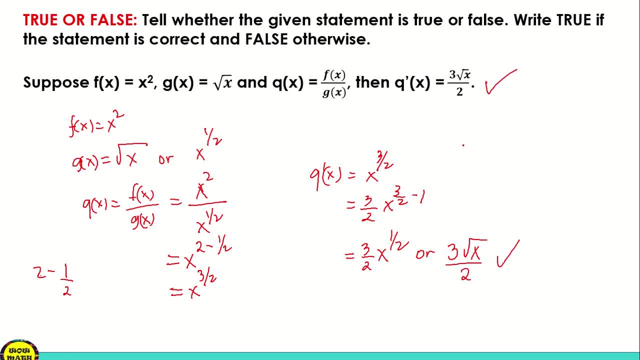 same sila nito. so therefore the statement is true. Okay, next tayo. So ano kaya ang derivative nung pupunin natin Yung, derivative daw ng X cubed times. the quantity of X squared minus 4 is 5X squared. 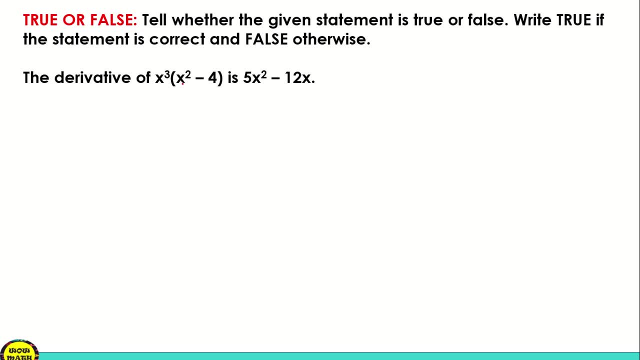 minus 12X. So check natin. So multiply muna natin. to. So X cubed times, X squared, that is X to the 5th power, X cubed minus 4,, that is 4X cubed. 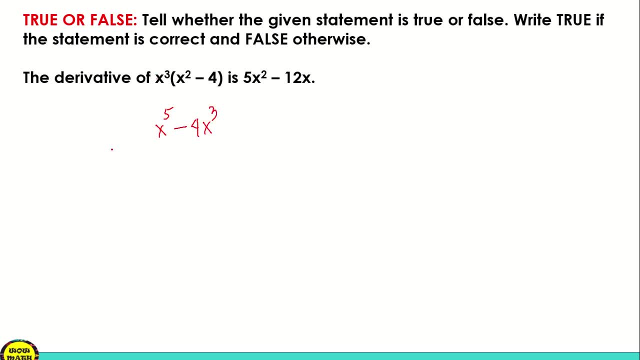 Okay. so kung punin natin yung derivative nila, so let's say, lagay natin as Y prime This is Y is equal to. okay, next, Pagkukunin natin yung derivative nila. so 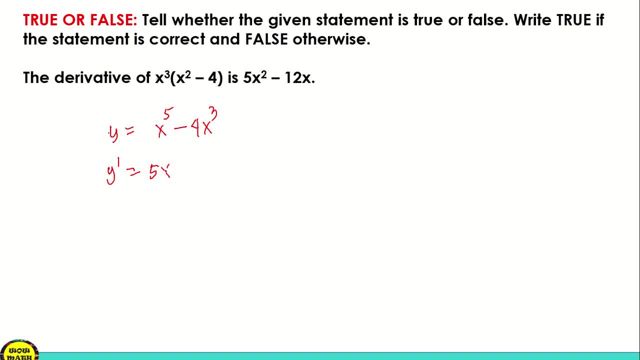 i-multiply natin yung 5 dito, So maging 5X to the 4th. Okay, minus 3 times 4 is 12X squared. So this is the answer. So kitang kita naman na hindi sila. 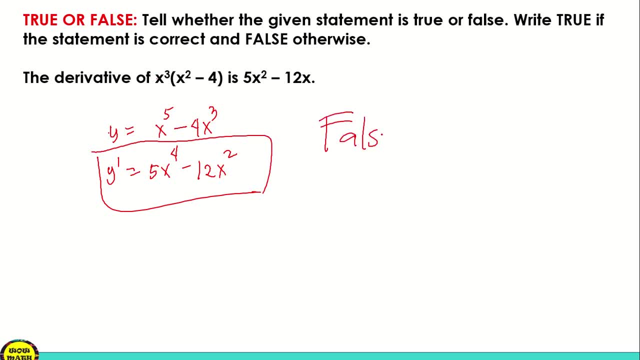 pareho. So therefore the statement is false. Next, if F of X is equal to the quantity of 4X squared plus 5X times the quantity of 2X squared minus 3X, then F prime of negative 1 is equal to negative 8.. So what? 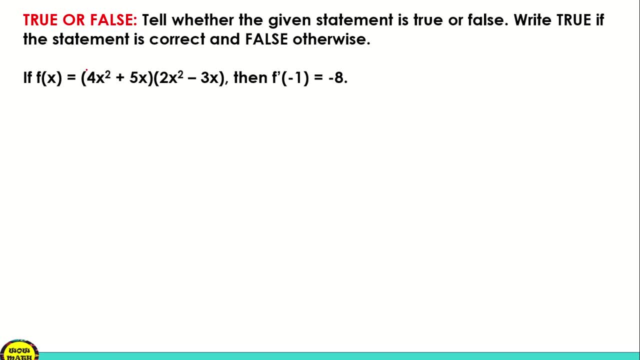 we're going to do subtract muna natin. So I multiply ito. So F of X is equal to pwede. foil method no: 4X squared times 2X squared, that is 8X to the. 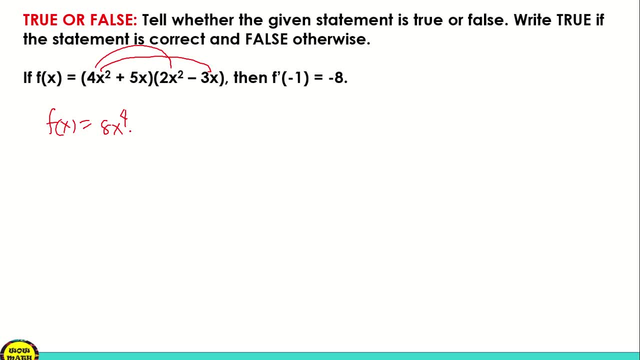 4th, So 5X times negative. 3X is negative 12X cubed. Next is 5X times 2X squared, that is 10X cubed 5X times negative. 3X is negative 15X. And then after that, okay, may makukumbine. 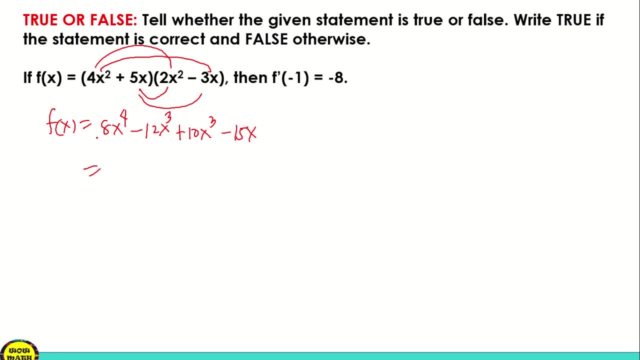 ba tayo Wala. So therefore, ito yung expanded form na Kukunin natin ngayon. ang derivative Okay F prime of X Is equal to 4 times 8, that is 32.. Bawasan ng isa, yung. 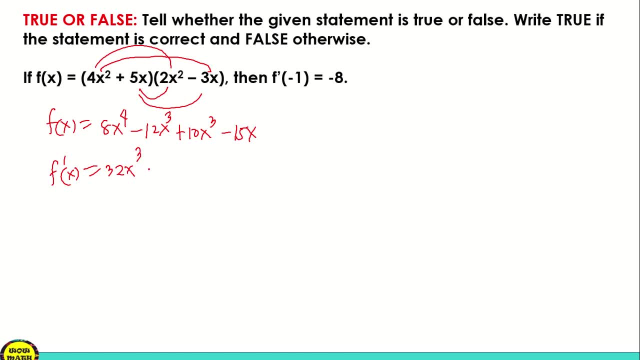 exponent: So X cubed na lang 3 times negative 12,, that is negative 36.. Okay, So that is 36.. So saan nga natin nakukuha yan 4 times 3, no, So negative 36X. 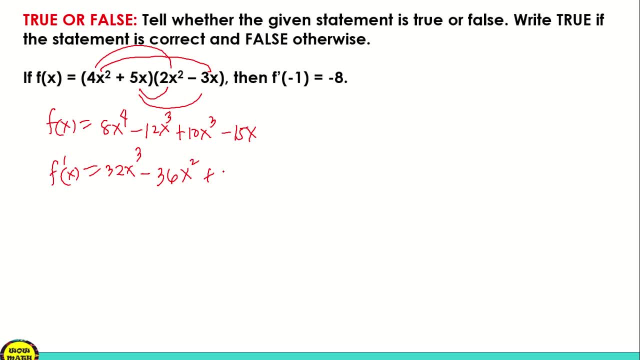 squared plus 30 X. Okay, So ano na. Okay, So hindi natin nakumbine pala ito, So dapat nakumbine natin. So i-double check nga natin yung sagot natin. We're going to double check. So this is 4X squared, Okay, So we're going. 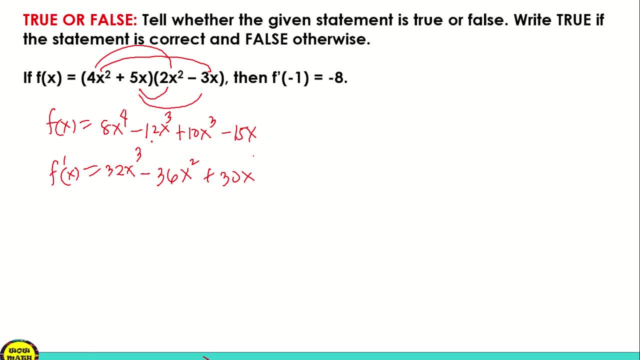 to double check first. no yung sagot natin. Okay. So dito class may kulang tayong squared Kasi 5X times negative, 3X, that is negative 15X squared. 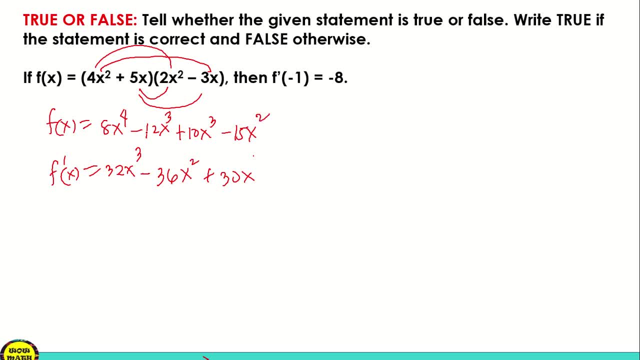 And then check natin: 8X to the 4th minus 12.. Okay, So 4 4X squared times, 2X squared, that is, 8X to the 4th 4X squared times. 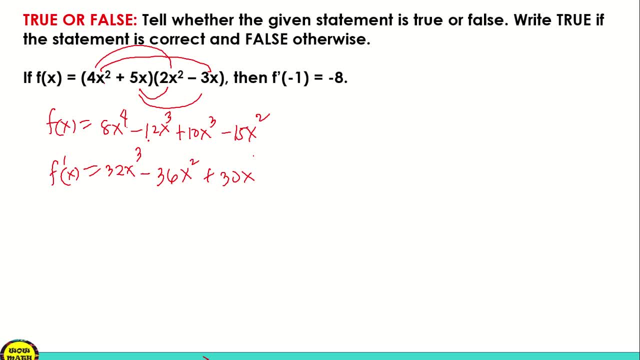 negative 3X, that is negative 12X cubed. Okay. And then yung isa naman 5X times 2X squared, that is 10X cubed minus 15X squared. So ito mali ito Okay. So tingin natin lang Ayusin, lang natin Mali ito, So brahin natin. 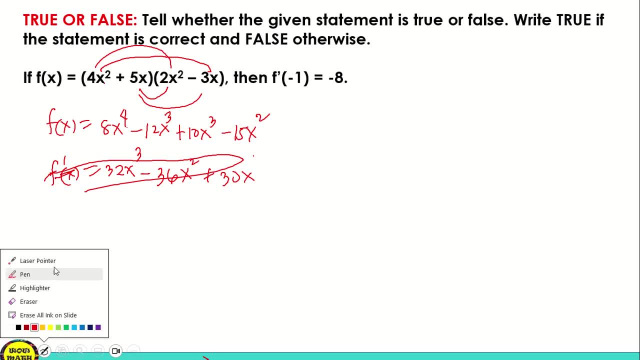 So again, kukunin na natin yun, no, yung derivative nya. So we have F prime of X is equal to 32X cubed. Okay, And then this one magiging okay, hindi pa natin. 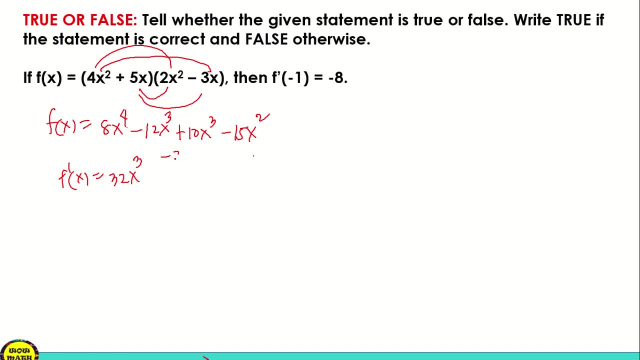 na add, So 12 plus 10, so that is negative 2X cubed. Okay, So ang sagot natin dito ay negative 2X cubed. Pagkukunin natin yung derivative that is negative. 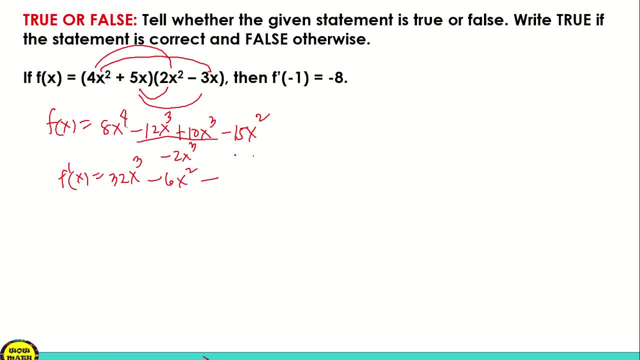 6X squared minus 2 times 15,, that is 30X squared, 30X. Okay. So since ang pinapakuwa ay F prime of negative 1, so i-check natin: no F prime of negative 1.. 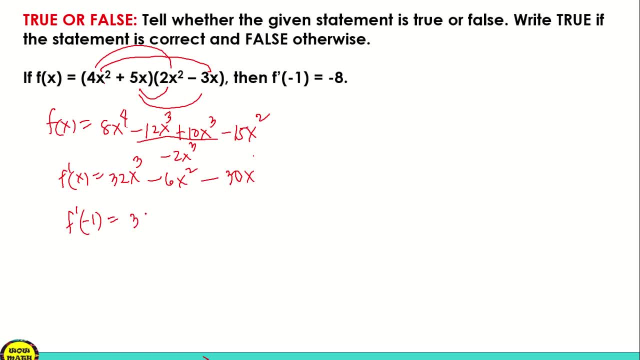 So palitan natin ng negative 1 yung mga X 32 times negative 1.. Okay, Cubed minus 6 times negative 1.. Okay, This is squared minus 30 times negative, 1.. Okay So. 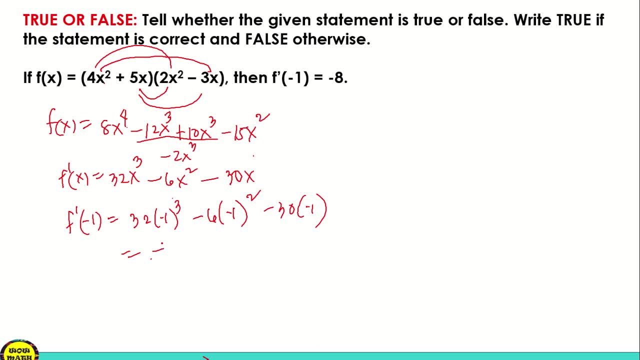 what is the answer Will be 32.. So this is negative 32.. And then, so this is negative 6 times, positive 1 and positive 30. Okay, So the answer will be negative 32.. Okay, Negative. 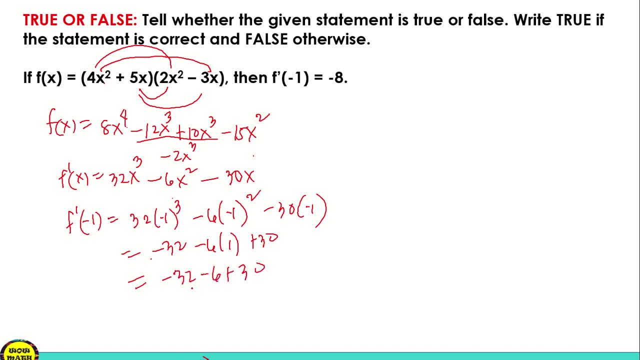 32 minus 6 plus 30. Okay, So negative: 32 minus 6, that is negative. what is that? Negative 26.. Okay, Negative: 32 minus 6.. So, if we cancel this, so negative: 32 minus 6.